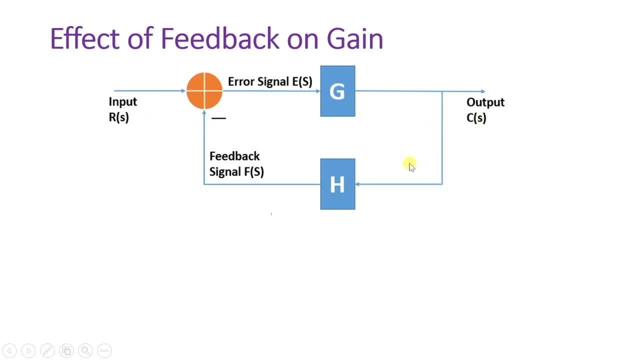 So, as per this feedback which is there with negative feedback- you can see by this negative sign I have placed negative feedback system over here. So, as per negative feedback system, we will be having transfer function of the system that we have already derived in my previous video. you can go through it For negative feedback transfer function, which 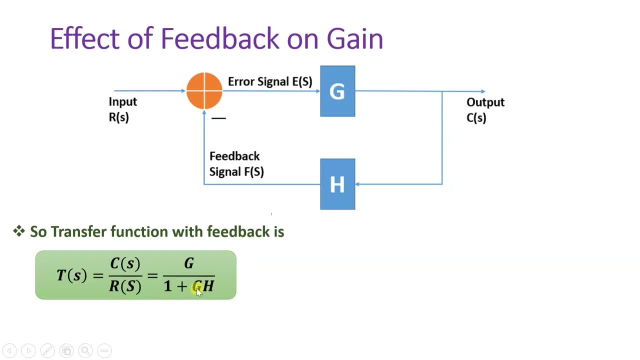 is CS by RS, that will be G divided by 1 plus GH. Observing, because of feedback, now your effective gain of the system, that will change and now that will get to G divided by 1 plus GH, If you observe gain of the system without feedback. 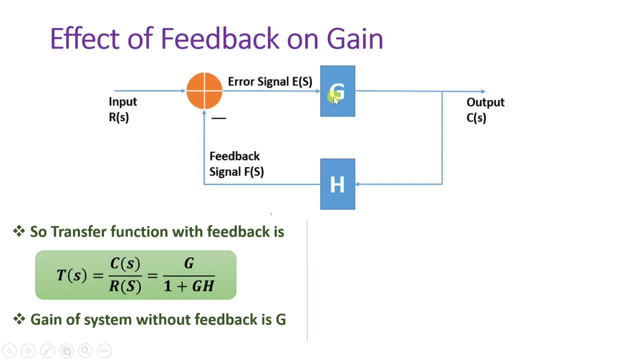 that is G. So this is my system. without feedback, its gain is G, but after feedback, with gain H, your resultant transfer function of the system that will translate it to G divided by 1 plus GH. So now you can easily observe. now your gain have changed. So what will be the effect that? 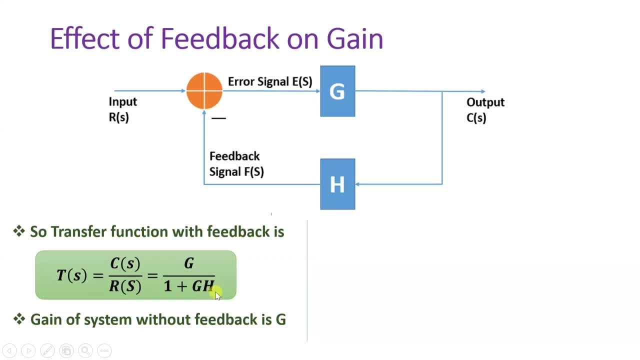 will happen on the system due to feedback gain H. So let us try to understand how it will effect to the transfer function. So here, as if you increase H, as if you increase H, this denominator, that is 1 plus GH, that will even increase, and as if denominator increases. 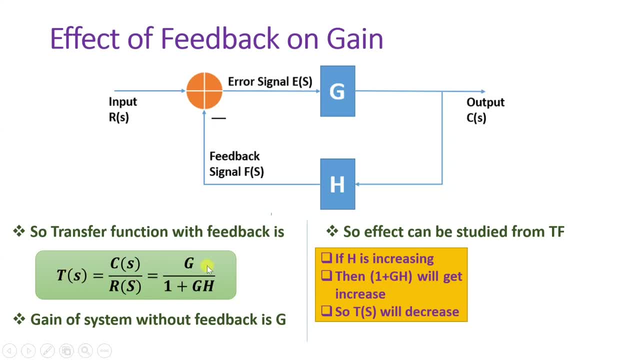 then resultant transfer function that will decrease, right? So if you increase H, then resultant transfer function will decrease. and if you decrease H then 1 plus GH that will decrease. it will result into increase in transfer function T of S. So because of feedback gain H there will be change in gain of resultant system where, as if we increase, 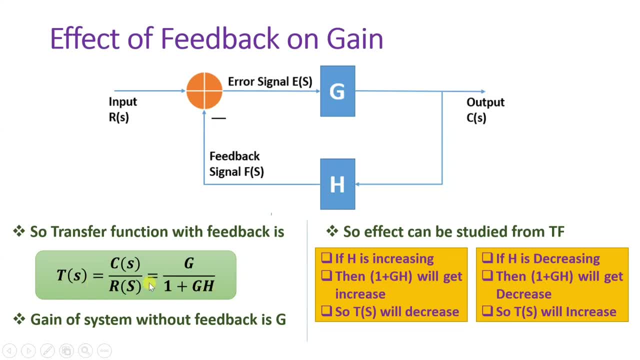 H, Resultant gain of system will decrease. and as if we decrease H then resultant gain of system will increase, right, But if you see overall gain of system, right, So overall gain of system due to negative feedback, that will decrease, that one can say Why the reason. 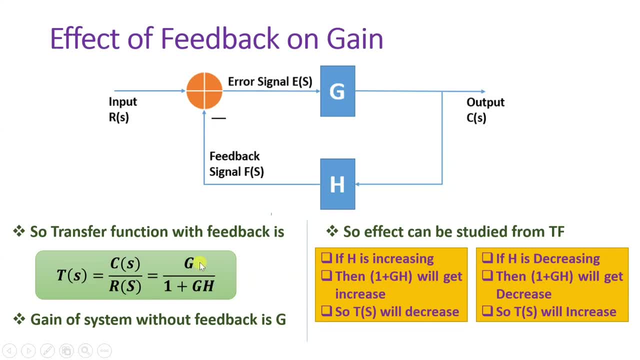 is as if you consider G is equals to 5 and H is equals to 1, then you just place that in this And 5 divided by 1 plus 5, so 5 by 6, that will be resultant gain. after feedback and without 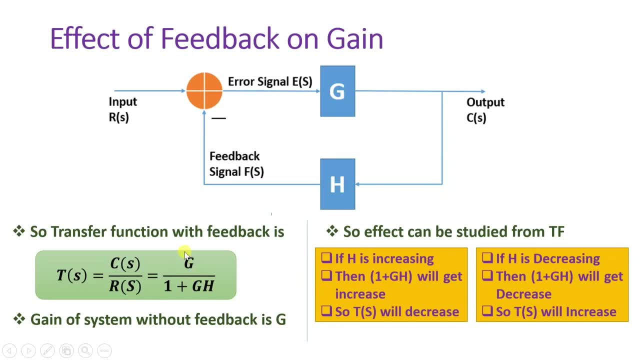 feedback gain is 5.. So resultant gain due to feedback will always decrease, but in with respect to increasing gain of H and decreasing gain of H, transfer function will change with its gain, as per the explanation which I have explained. So we can say: by changing H we 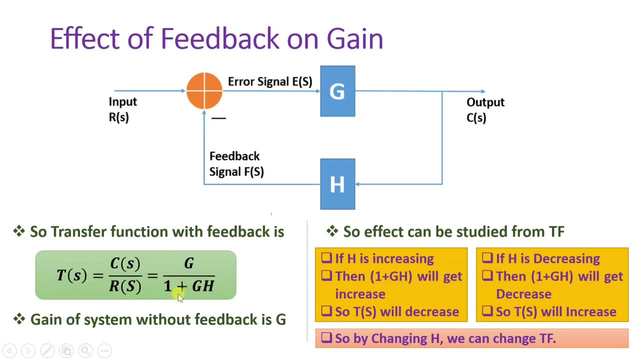 can change transfer function due to feedback right. So that is how effect of feedback is happening on the gain of the system. For positive feedback, your transfer function will be G divided by 1 minus GH right, and as per that, you can understand this explanation. 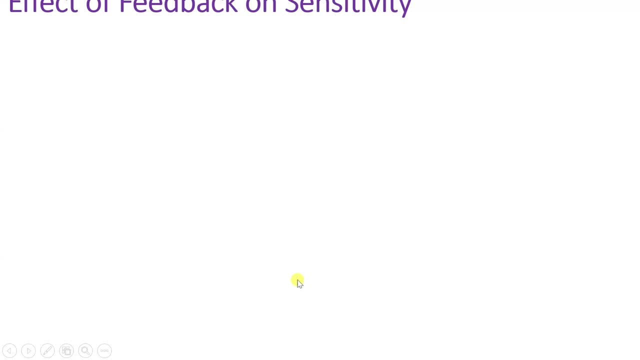 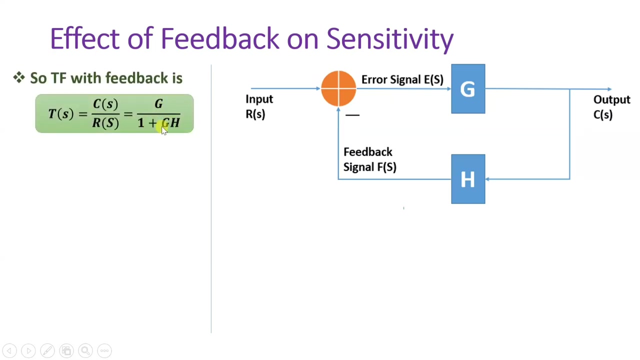 Now let us move on to second point, that is, effect of feedback on sensitivity. So here we are, considering same system with negative feedback and, as per this negative feedback, your transfer function, that will be g divided by 1 plus gh. Now, first of all, we need to understand what is sensitivity of the system. 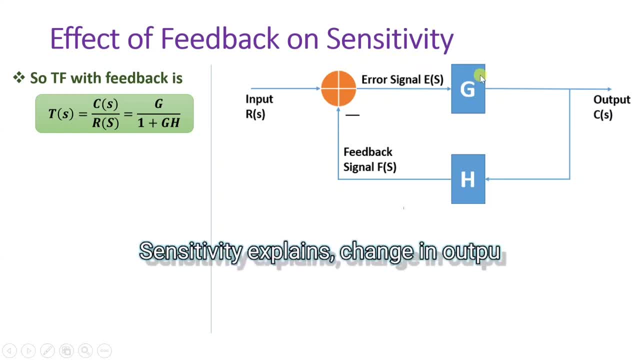 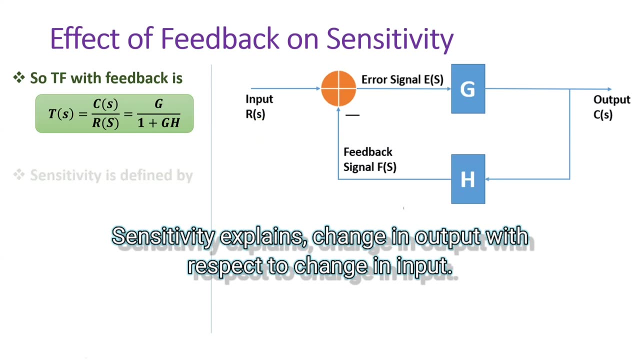 Now see. sensitivity explains how much change happens at output side with respect to change in input. If change at output side is larger with respect to change in input, then one can say our system is more sensitive. and to understand what is sensitivity, the basic function is percentage. 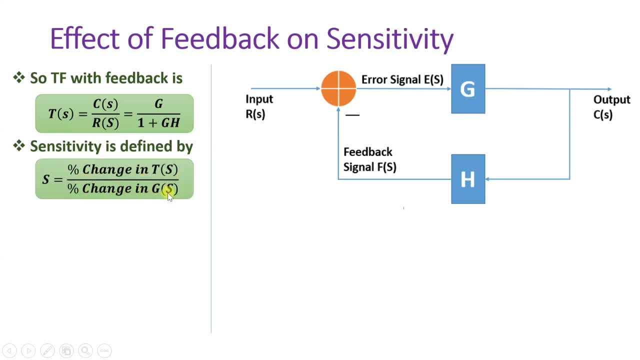 change in transfer function divided by percentage change in gain of the system. Here transfer function is T of s, that is g divided by 1 plus gh, and gain of the system, that is g. Here in suffix I have written s means it is there. in Laplace domain one can write only: 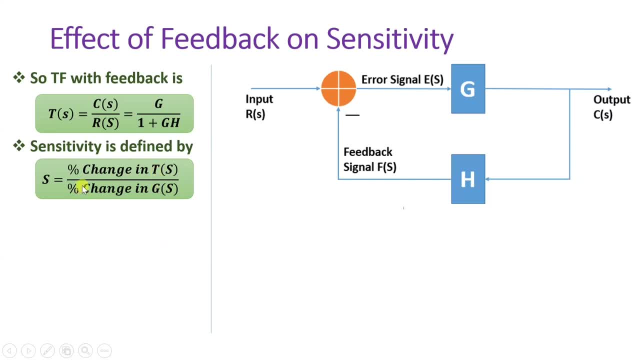 g or only g? Now, what is percentage change in T of s? Percentage change in T of s is dt by T into 100 and percentage change in g, that is dg by g into 100. And if you further simplify this, then this 100 will get cancelled and this sensitivity. 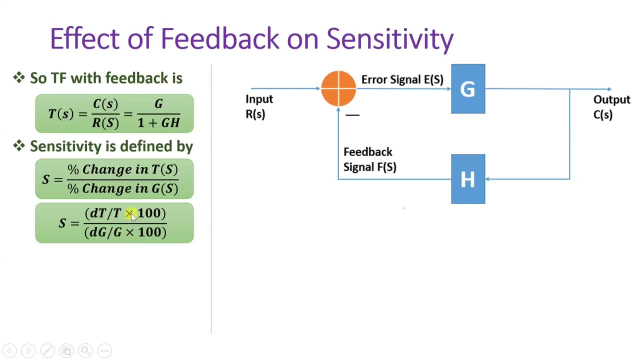 will be dt by dg into this g will go in numerator and this t will go in denominator, so that sensitivity will be dt by dg into g by t. So this is my sensitivity, right in terms of formula, And, as I have told you, sensitivity is what it is. change in output with respect to change. 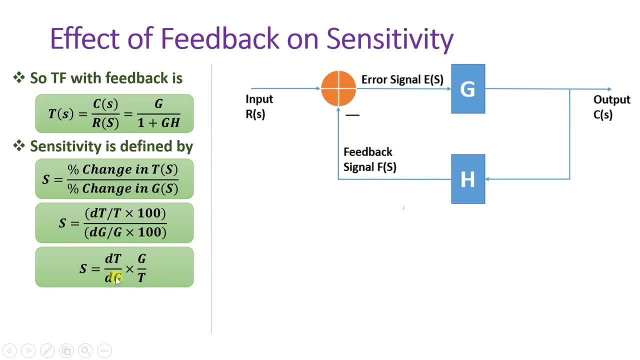 in input and in terms of function, we can say it is dt by dg into g by t. Now let us try to derive this function and at the end we will conclude how sensitivity will change, How sensitivity will change with respect to feedback gain. h. 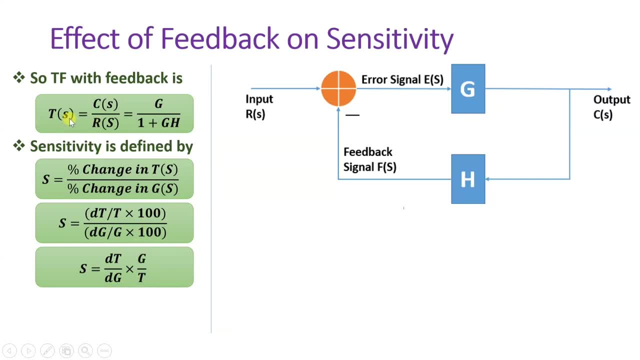 So to have g by t we can use this transfer function. T of s is equals to g divided by 1 plus gh. So here we can say: g divided by t, that is 1 plus gh. You see, we are just taking this 1 plus gh term over this side and t term in denominator. 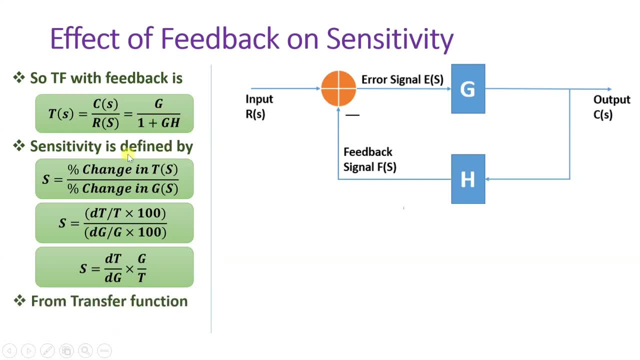 of g. So from transfer function we can say: g divided by t. So we can say: g by t is equals to 1 plus gh. as per this transfer function, Now we have g by t and now we need to derive dt by dg and if we place that in this formula, 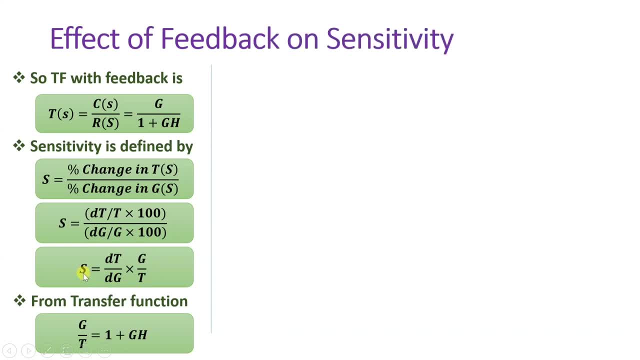 we can have resultant sensitivity. So here, to have sensitivity, we need to have dt by dg. and to get dt by dg now we will differentiate this t with respect to g, So dt by dg where t is g divided by 1 plus gh. So here we are differentiating this t with respect to g. 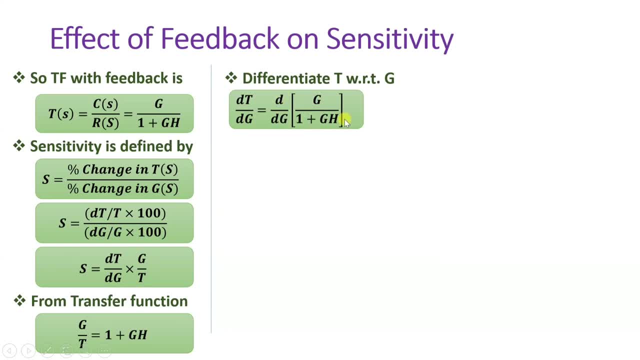 Now, you see, this is what differentiation of g divided by 1 plus gh. So here we need to apply division rule of differentiation. So what is the division rule of differentiation? it is denominator term into numerators, term differentiation. So you see, this is the division rule of differentiation. 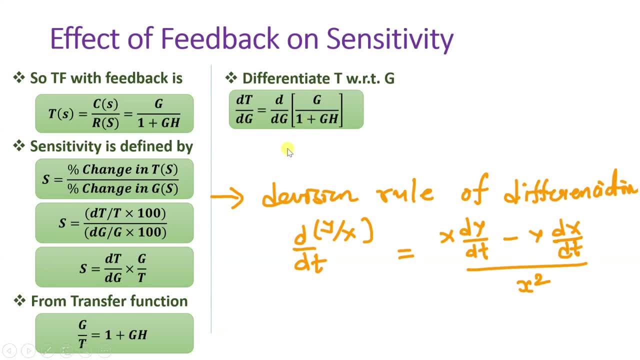 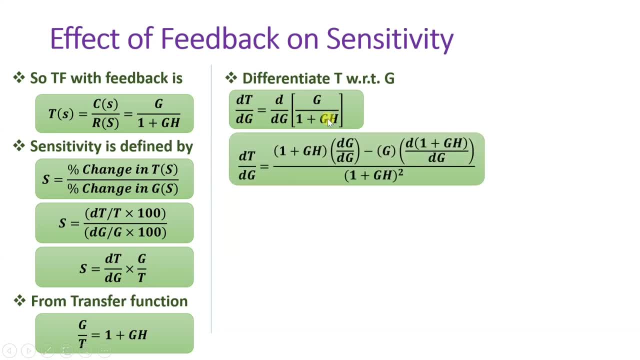 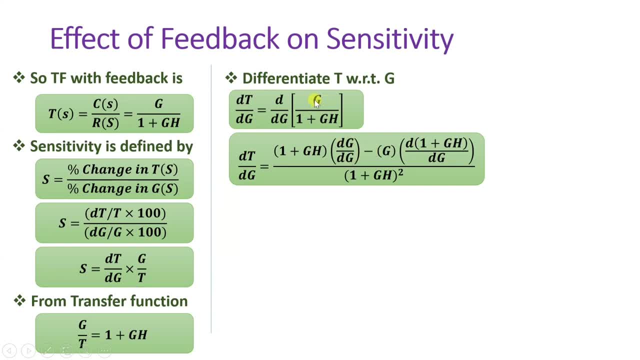 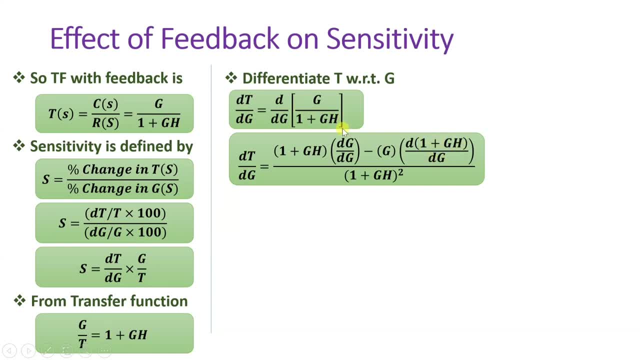 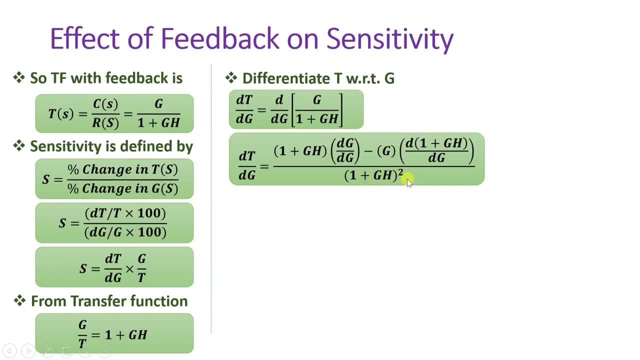 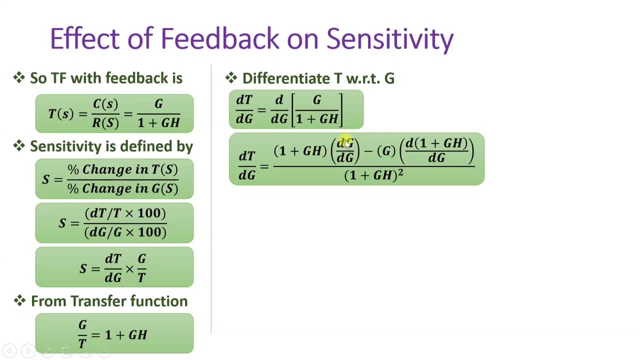 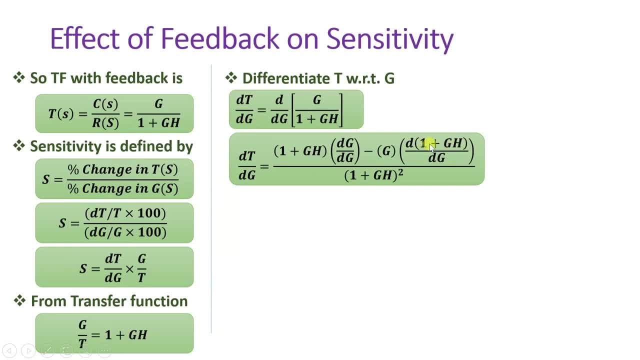 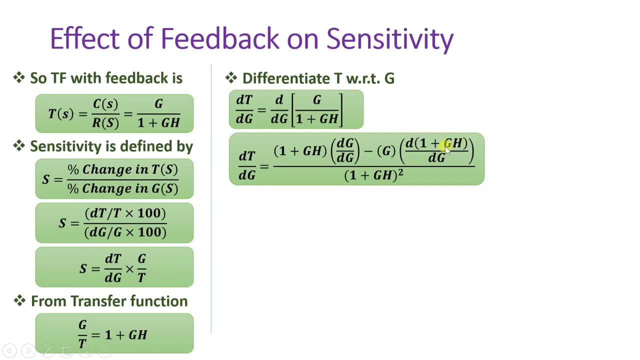 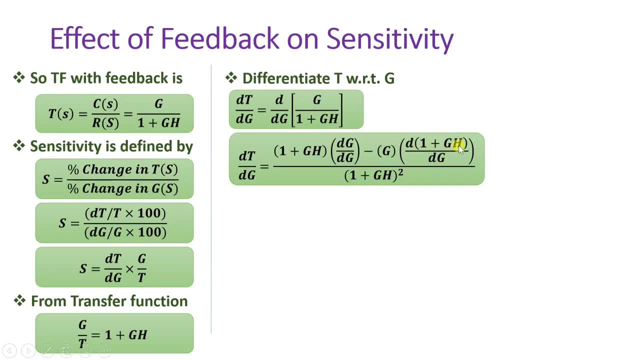 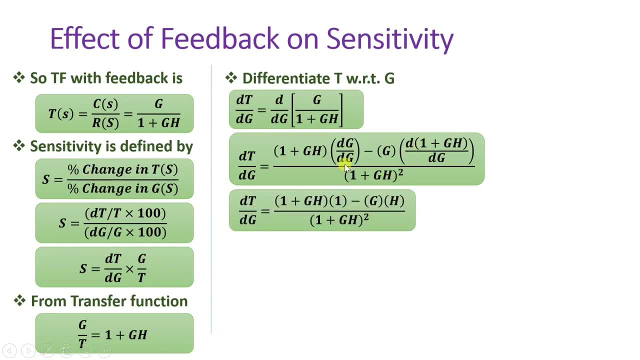 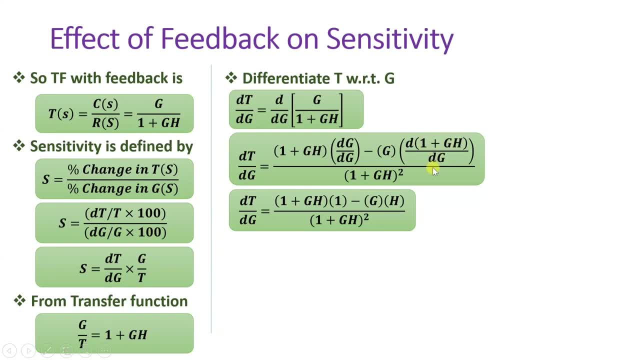 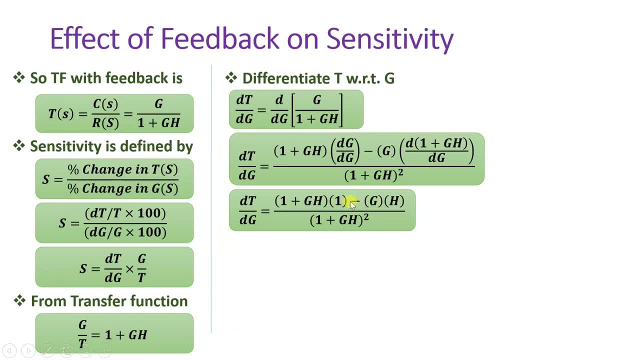 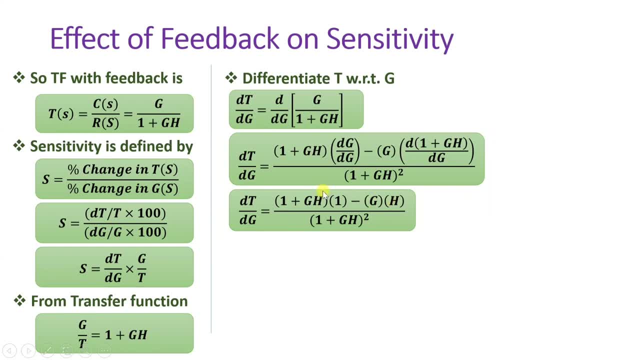 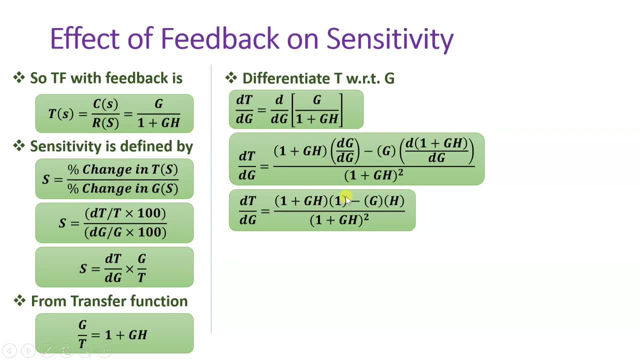 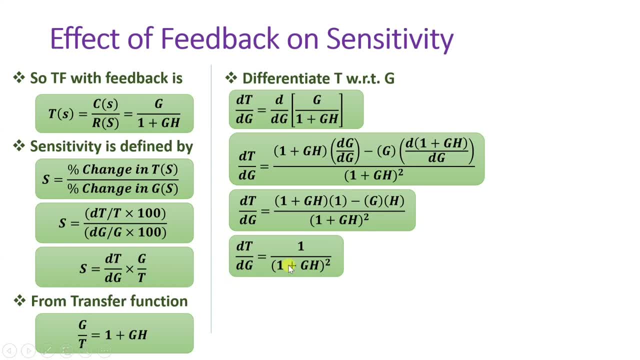 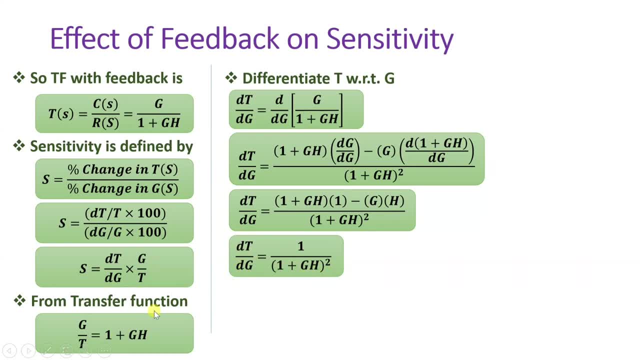 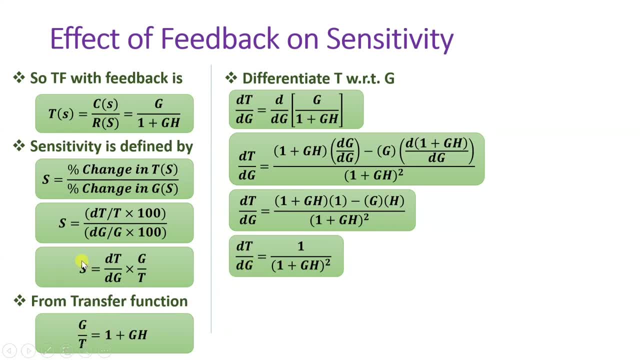 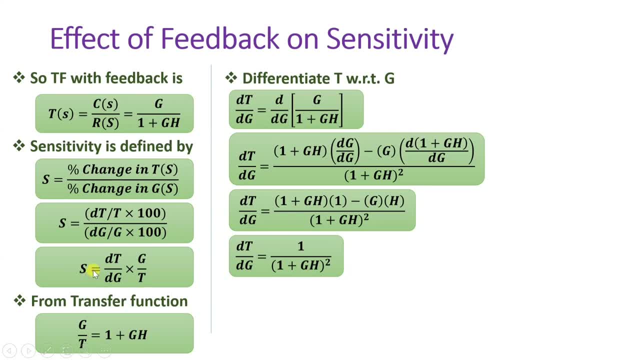 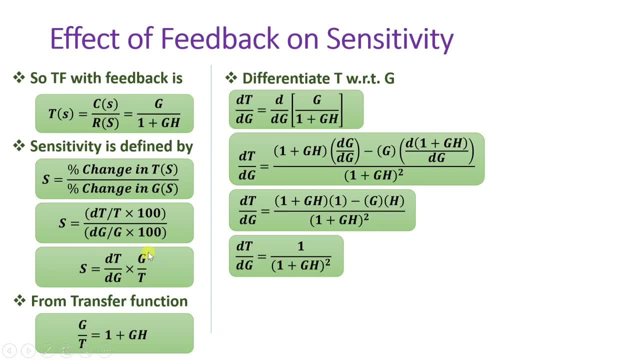 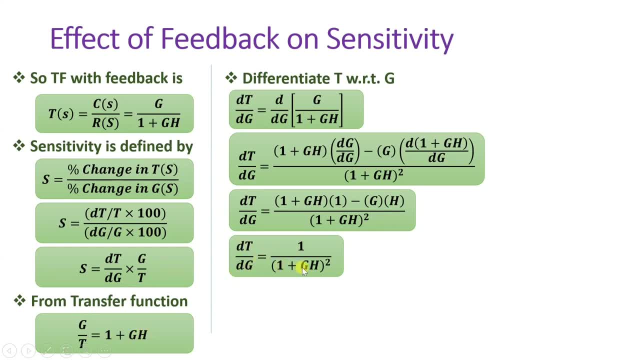 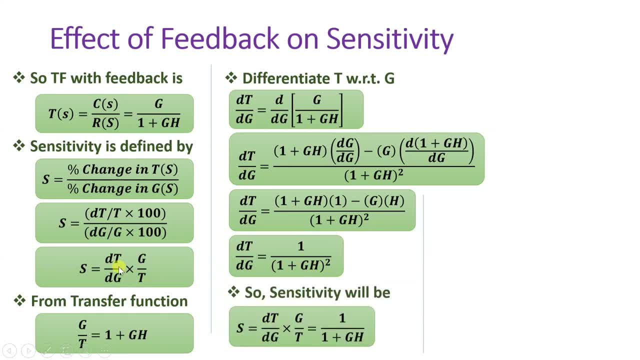 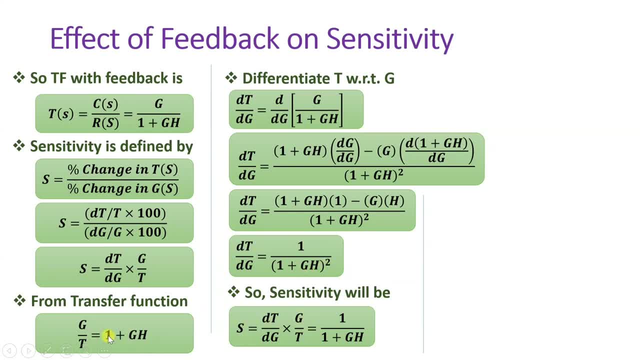 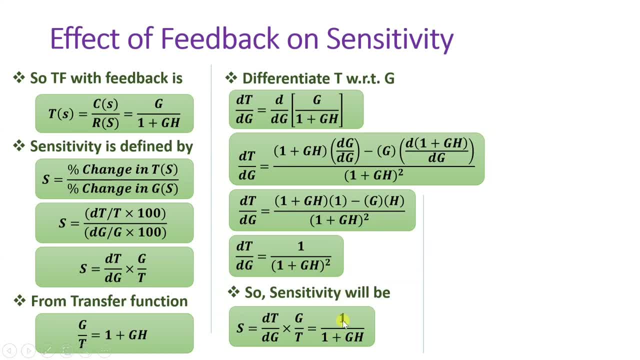 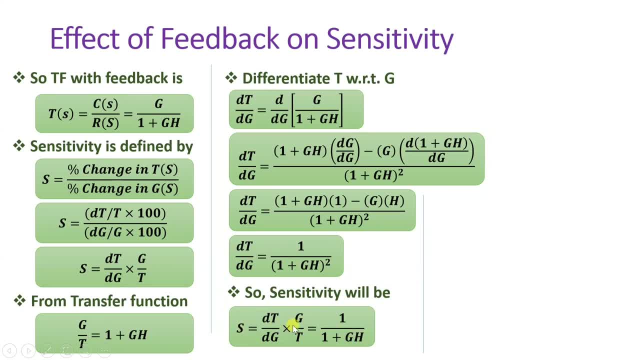 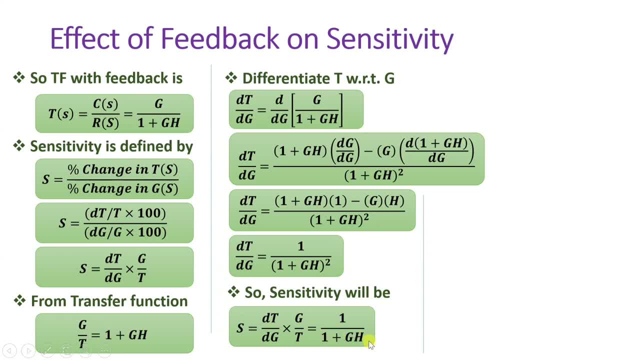 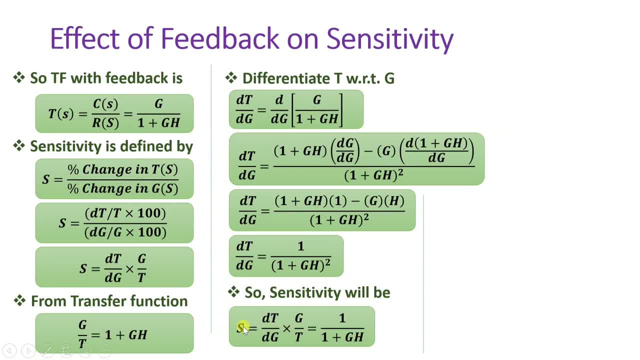 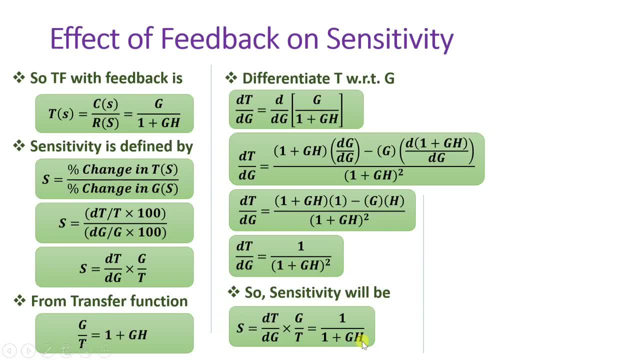 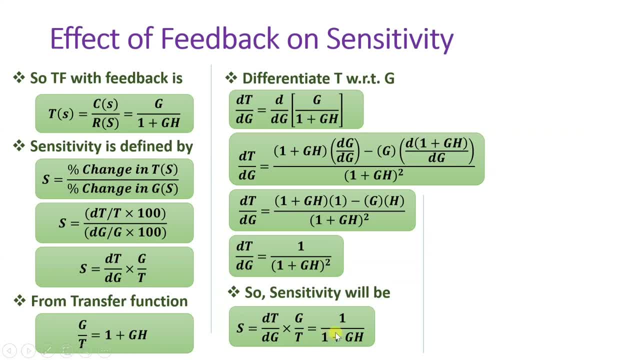 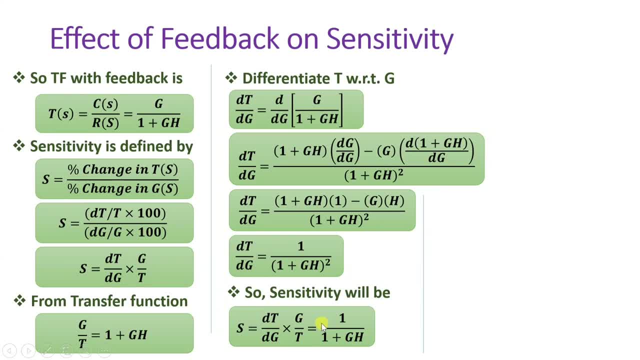 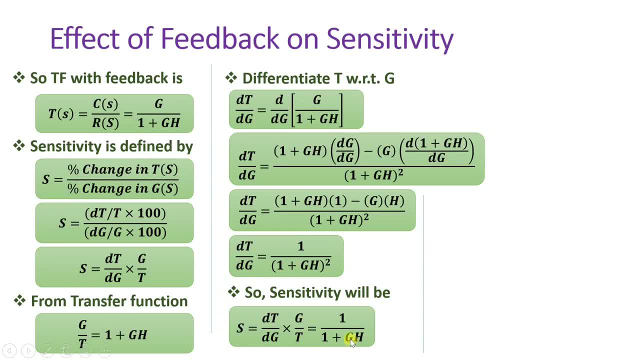 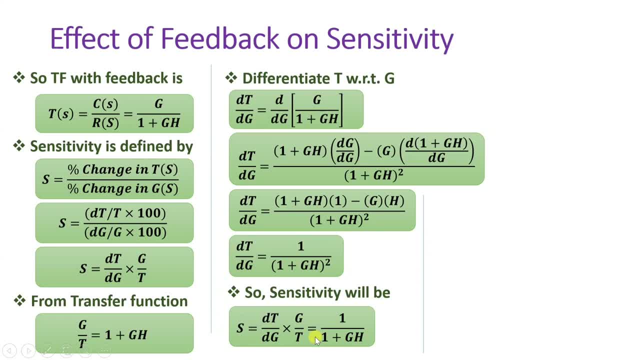 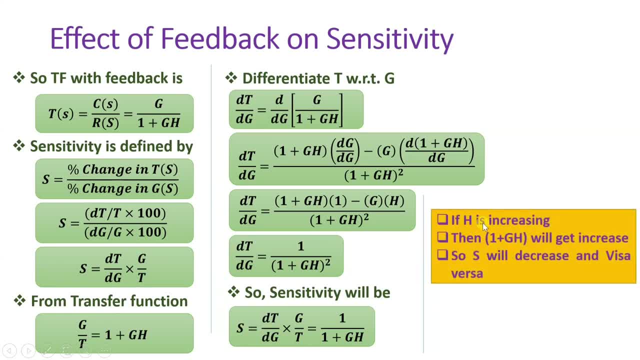 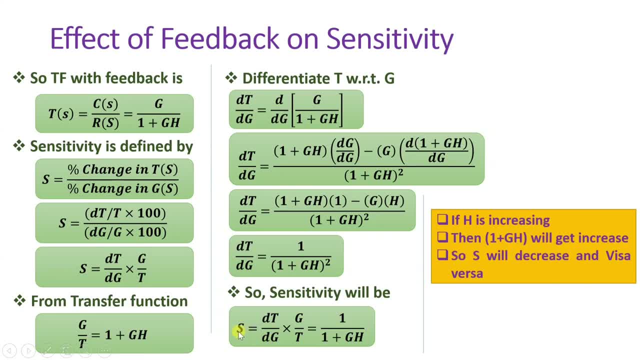 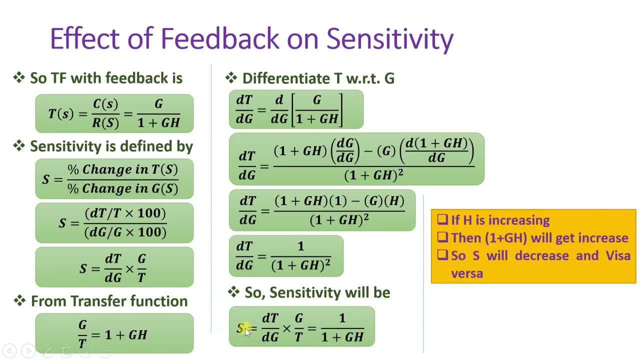 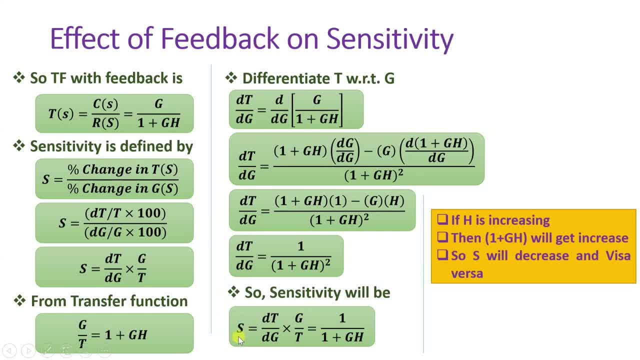 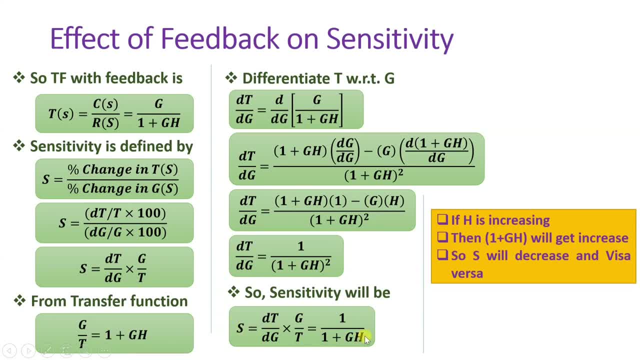 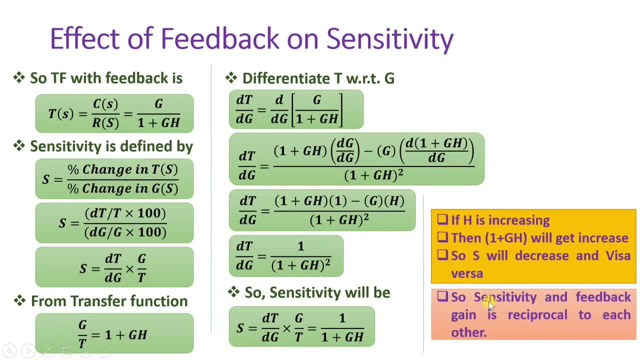 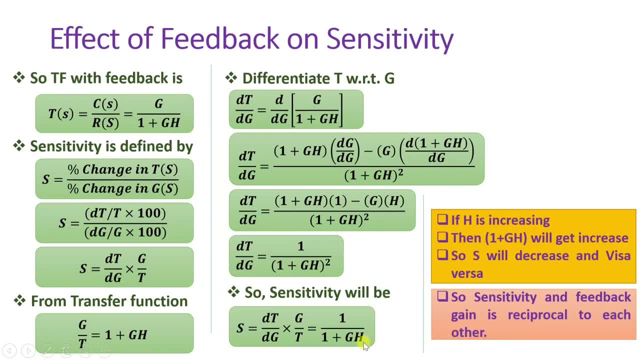 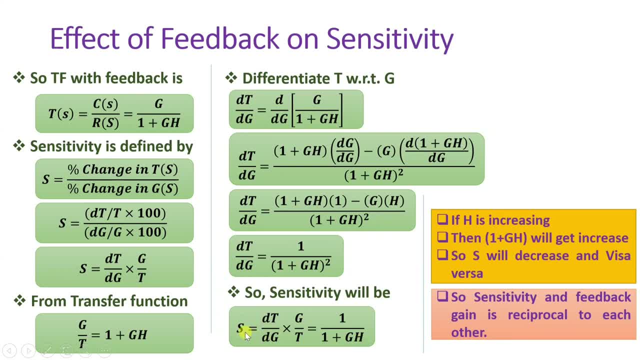 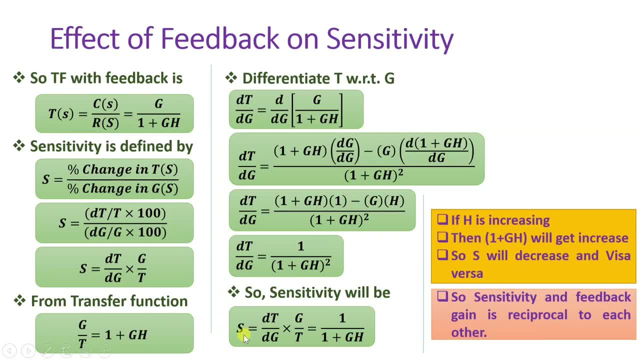 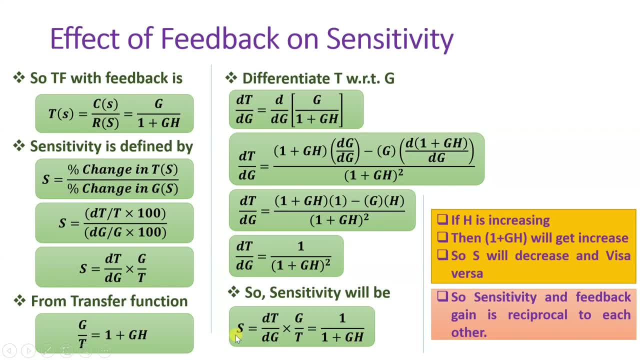 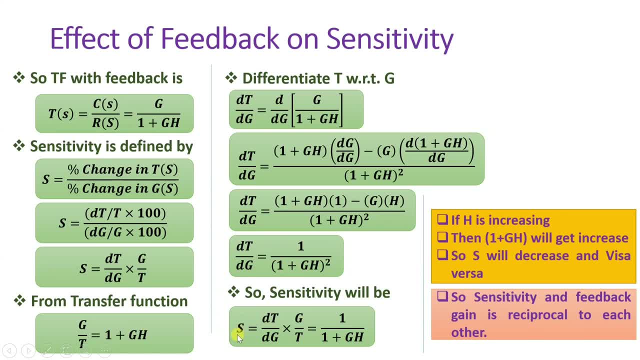 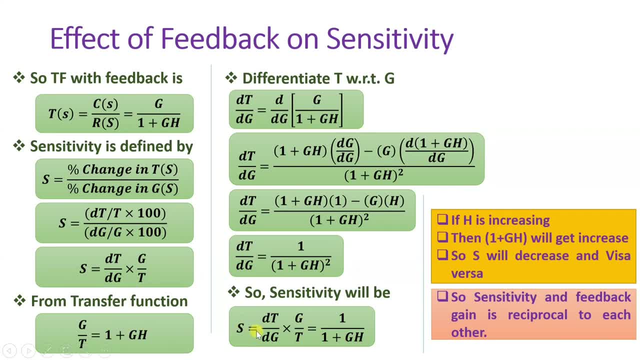 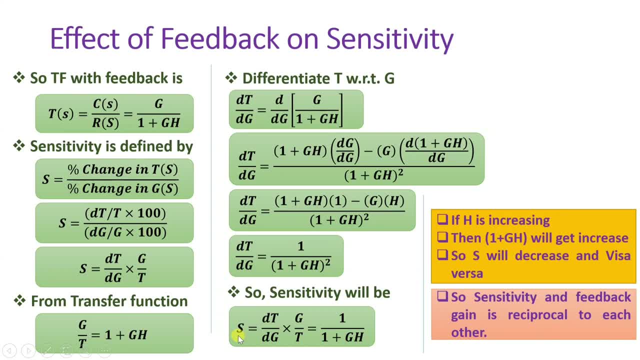 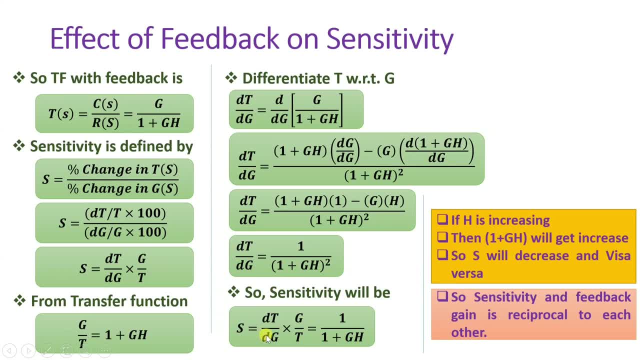 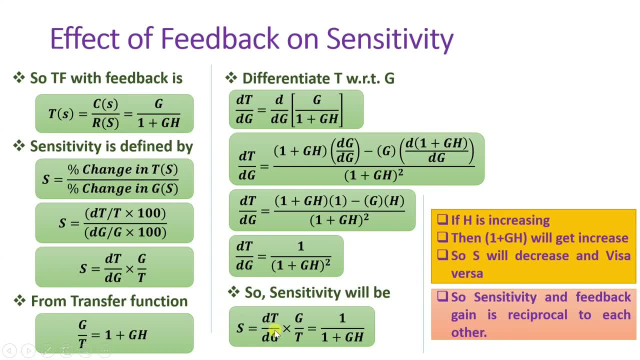 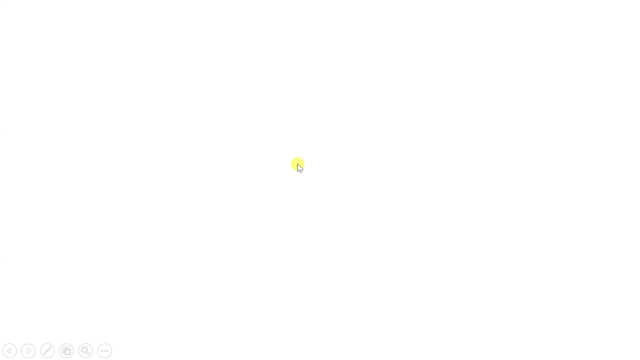 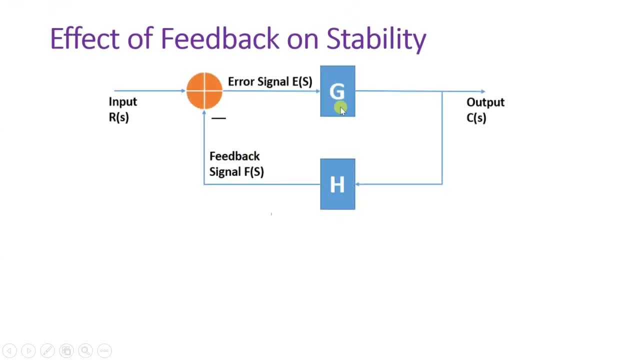 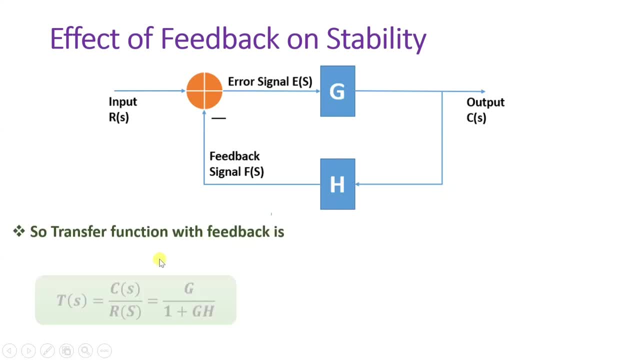 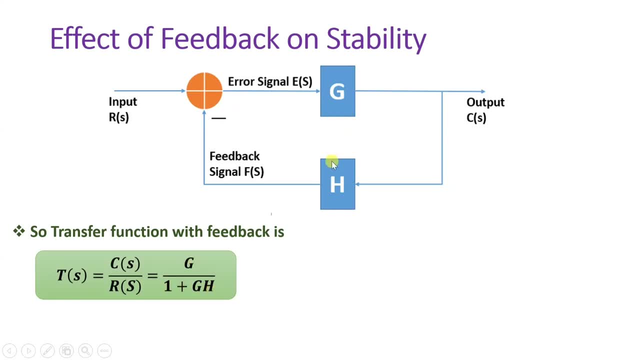 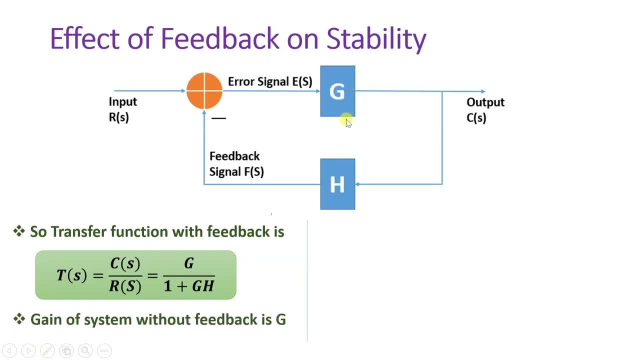 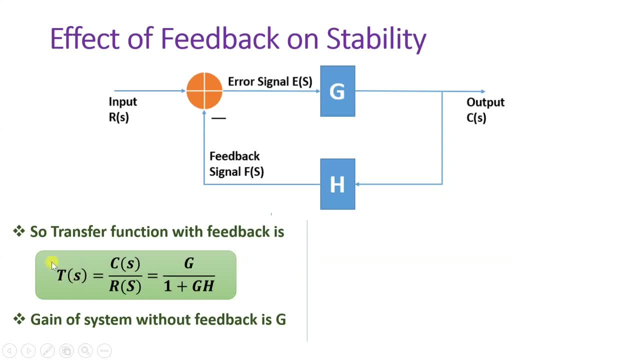 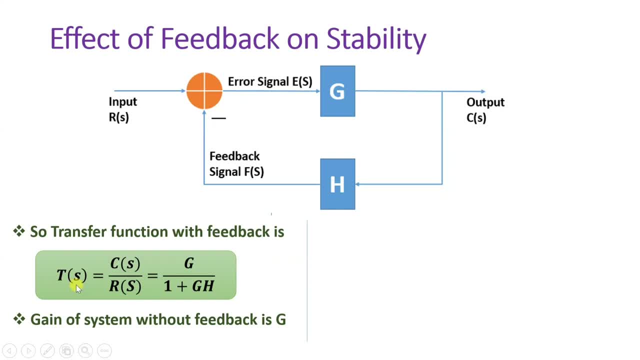 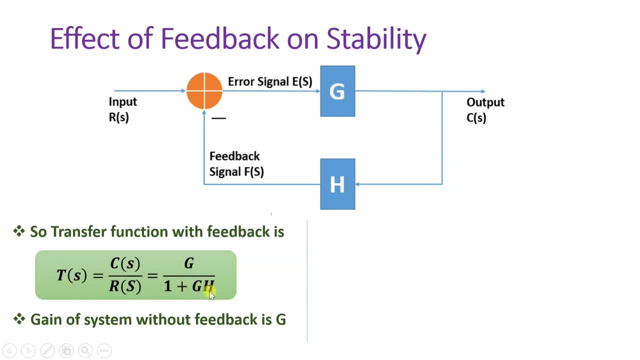 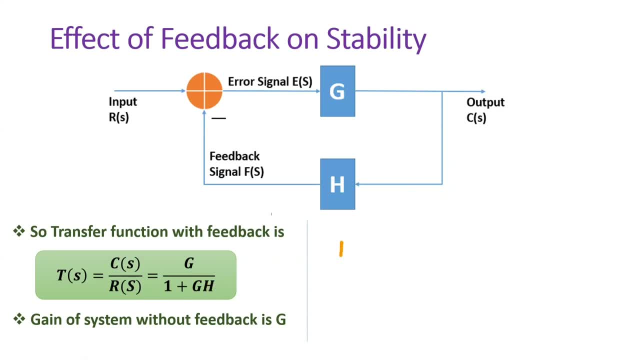 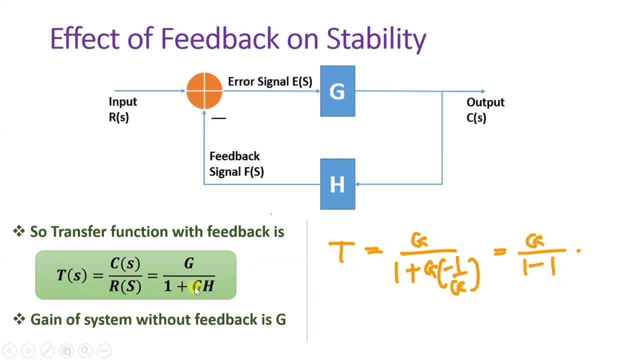 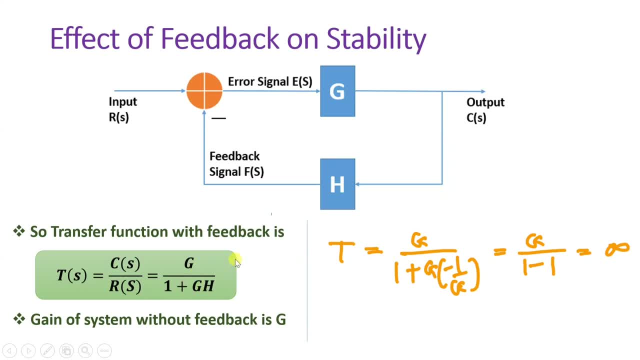 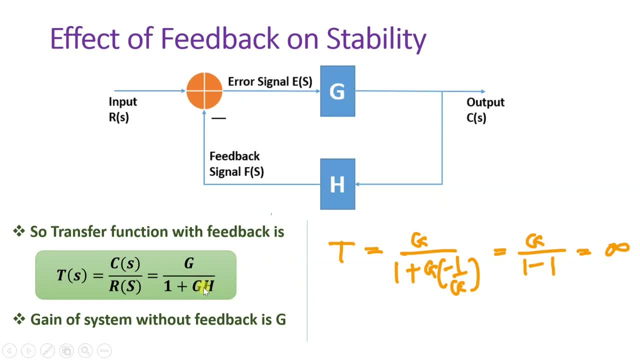 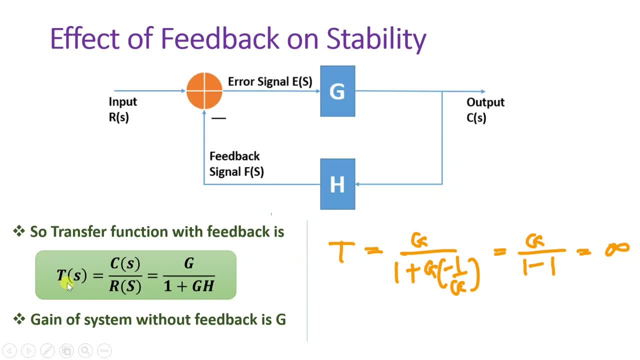 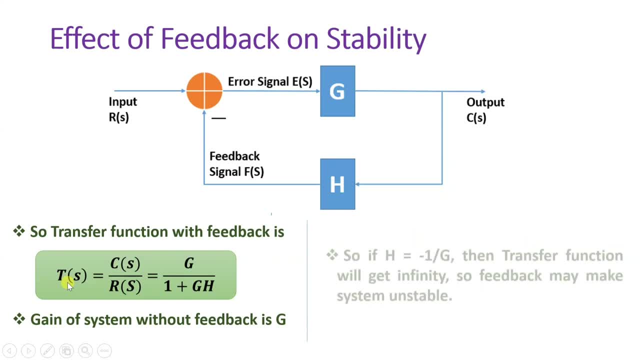 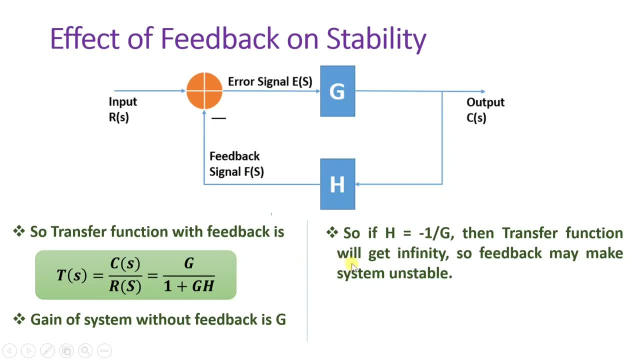 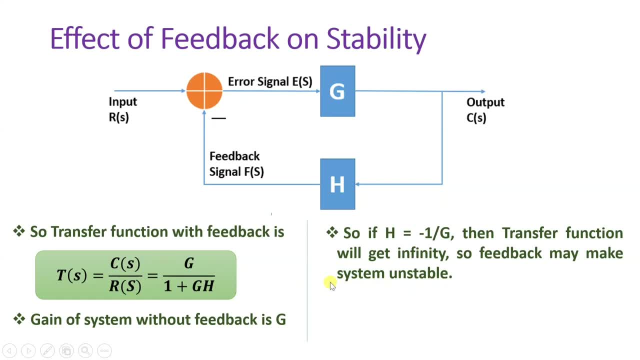 so feedback may make system unstable. right, and you will be finding always open loop. system is stable in most of the situation, but due to feedback it may result system unstable. right, and same case that may happen for positive feedback. so due to feedback, stability of system decreases. right that one can conclude. so this is how effect of feedback is there on gain? 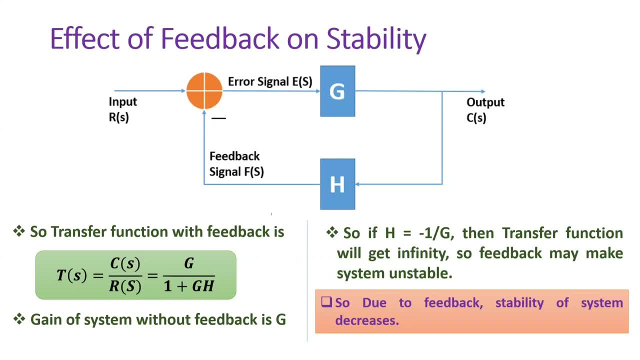 on sensitivity and on stability. i hope that you have understood this video. thank you so much for watching this video. please do give your valuable suggestions. the reason is your suggestions are motivating me and, based on your suggestions, in future i'll make videos which will be resolving your queries. thank you so much for watching this video.